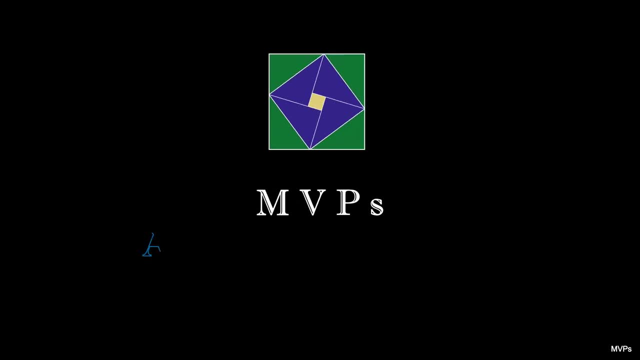 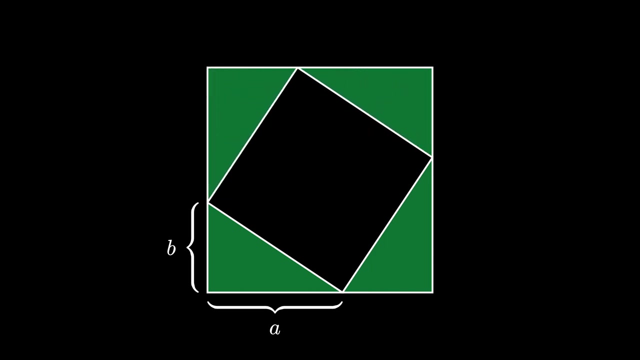 What do these diagrams have to do with the arithmetic mean, geometric mean, inequality? Let's find out. Start with a right triangle with legs of length a and b. Use four copies of the triangle rotated so that we create this shape, which is a square with a side length of a plus b. Inside there's a missing square. 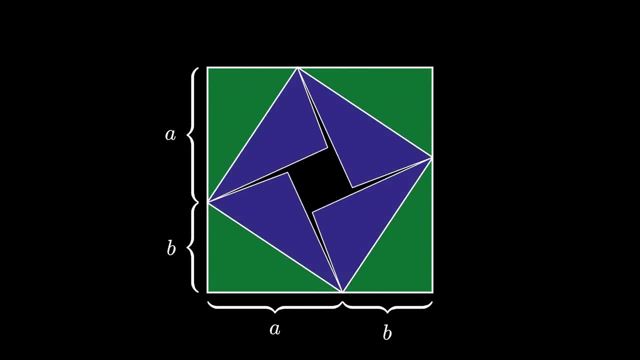 Reflect each triangle about its hypotenuse, creating this diagram using eight triangles. Notice there's still a missing square inside. To verify that this missing inside shape is a square. notice that the side length can be computed as the difference of the leg lengths of the original triangle. So we 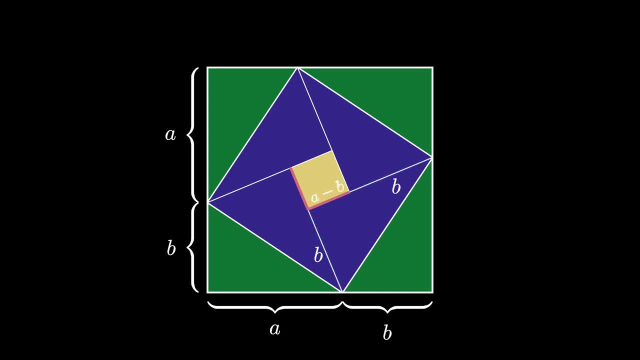 see that this is a square. Next we'll verify that the side length is a point in the triangle. this square has a side of length a minus b. Now we can find the area of this shape in two different ways. First, we note that it is an a plus b by a plus b rectangle, so the area is a plus b. 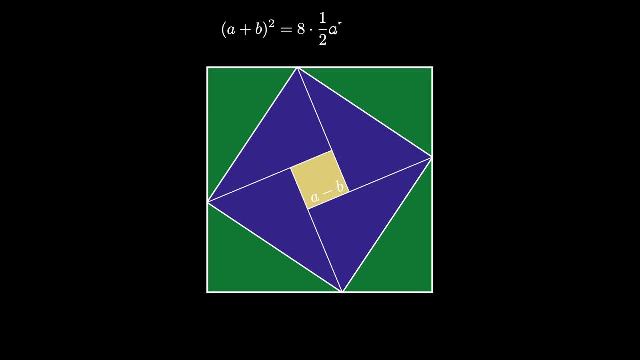 quantity squared. On the other hand, we've used 8 triangles plus the inner square, so we have an area of 8 times a half ab plus the quantity a minus b squared. We can simplify the 8 triangles to have the area 4 times a times b. 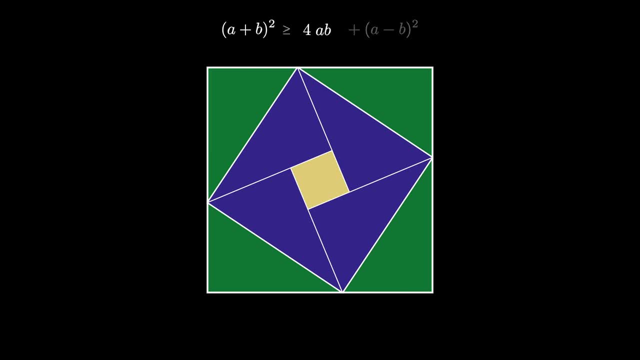 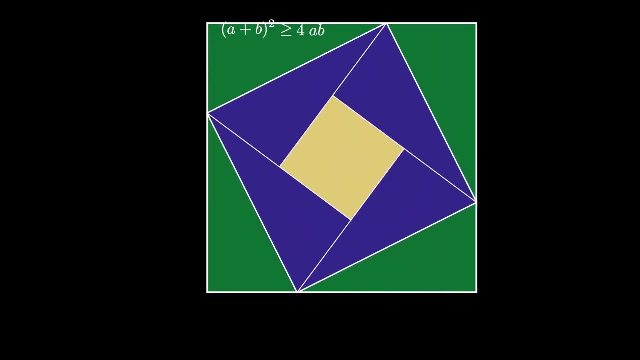 Now we note that the quantity a minus b squared is always non-negative, so if we leave it off, we obtain the inequality. a plus b squared is greater than or equal to 4 times a times b. As we vary a and b, we see that the inner square gets larger and smaller, depending on. 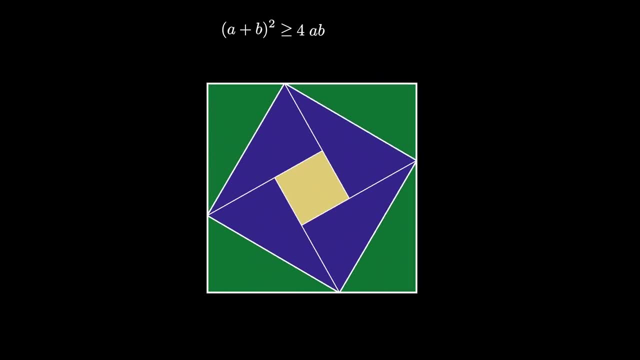 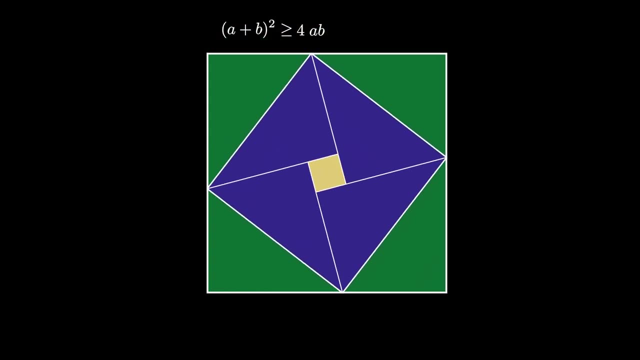 the sizes of a and b, but we also note that the square is always there, except in the one instance when a and b are exactly the same, so that that square shrinks to 0 area. From this we conclude that we have equality amongst the inequality and we have equality. 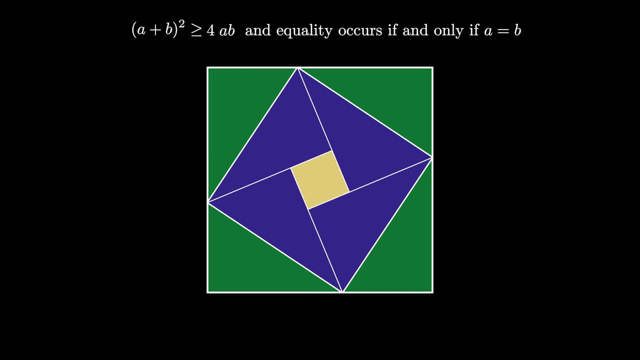 if, and only if, a minus b is 0, so that a equals b. Upon taking square roots and dividing both sides by 2, we obtain the inequality: a plus b over 2 is greater than or equal to the square root of a times b. This is the arithmetic mean, geometric mean: inequality.